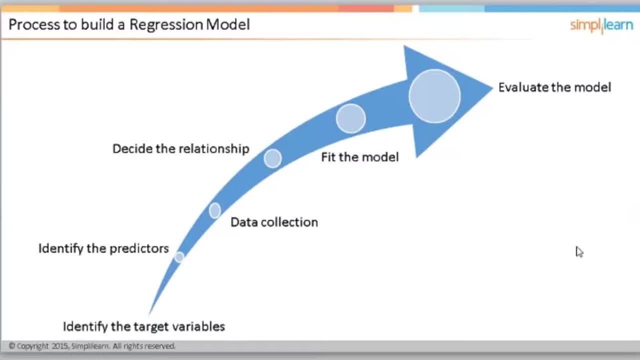 that is the purpose of this particular linear regression, because linear regression is a model which is based on all the x parameters. So even for future, if you are, if you want to predict your future y value, you need to know what are all the future x that you are. 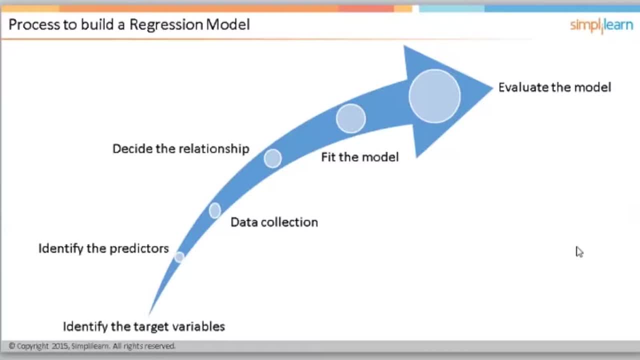 going to do. ok, In that case. if, if you do not have factors to represent it, then why? ah, only then time series come into the picture. So that is what we are going to see today. what is time series? because time series does not require any any factors to be represented. ok, Clear. 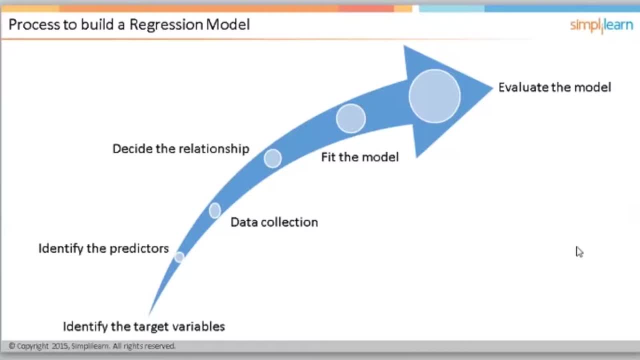 Sanal. ok, great, I. I said like k-means clustering and ah in k-means clustering. as I said, you would know what is the cluster size that you want to form Initially. if you, if you are trying to form three clusters, your cluster seeds would be three. It would select three. 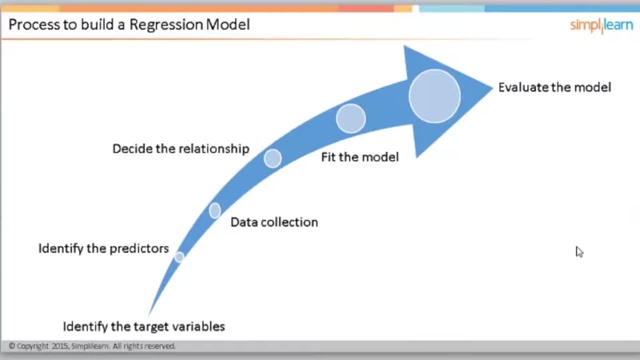 three random sheets based on the distance. it tries to group all this data points and it will form the cluster. So this iteration would happen until none of your data points move into the other cluster. So this this process happened and in, if you are looking. 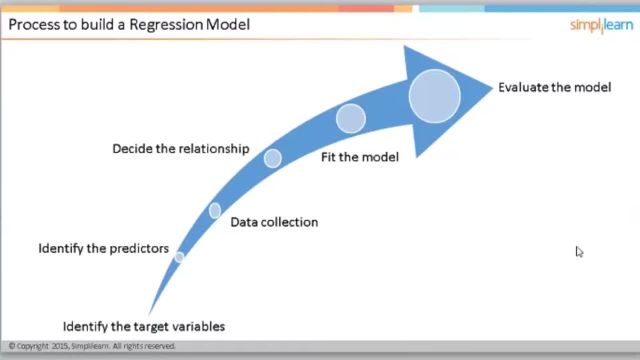 at hierarchy clustering. hierarchy clustering is also a process where, based on the minimal distance, it tries to club together. So hierarchical is something from a big cluster you are trying to categorize into two different clusters. So if the distance are more, those data, those 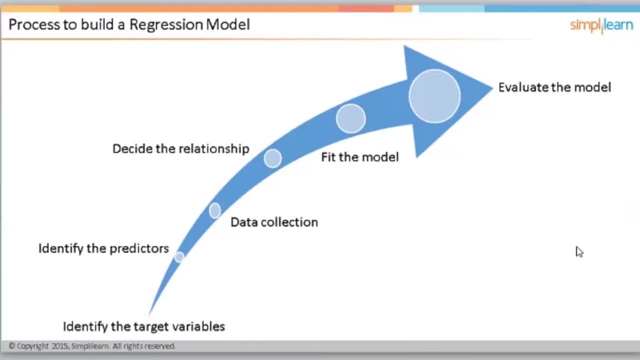 data points are separated and an individual cluster is formed. So this happens until it is divisive. So at some point of time it cannot be divided further, So it stops at that particular point. that is called hierarchical clustering. So probably what we will do is: 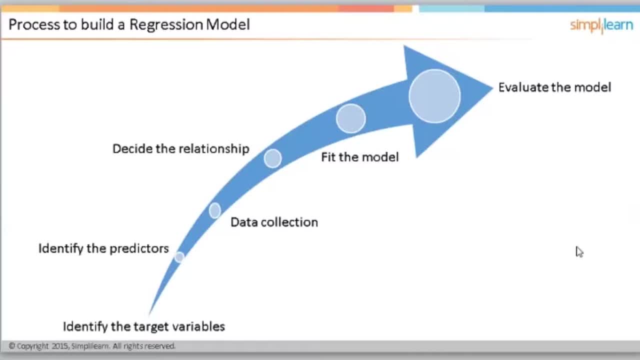 today we will just start with time series, and tomorrow I will get into a case study where we will try to solve all the clustering techniques and time series as well together. ok, fine, So we will start with time series, Because in clustering I think I did not give any example for hierarchical clustering. So 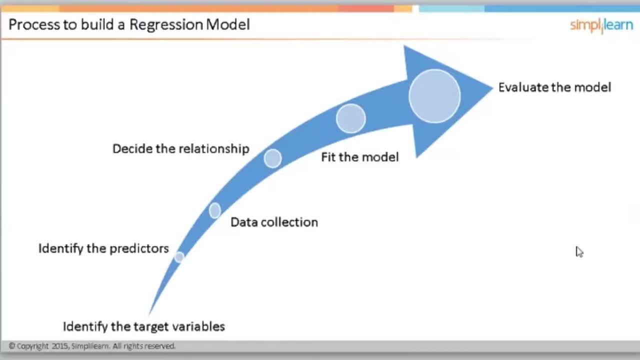 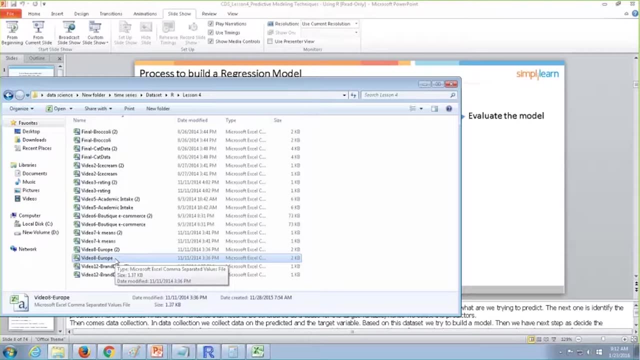 I will show you some of the examples in hierarchical clustering first. then I think we can start with the process. meanwhile I will just check what sort of data I have. probably right now I will just try to take this data set and I will tell you how hierarchical clustering. 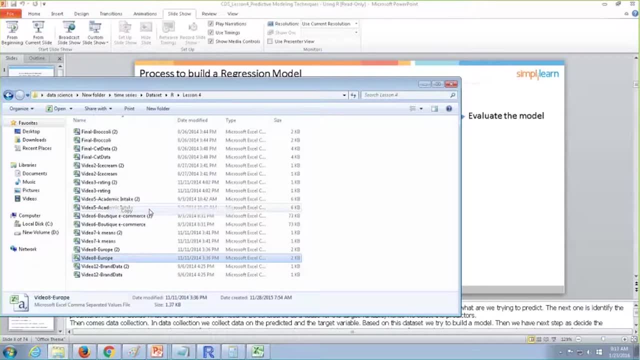 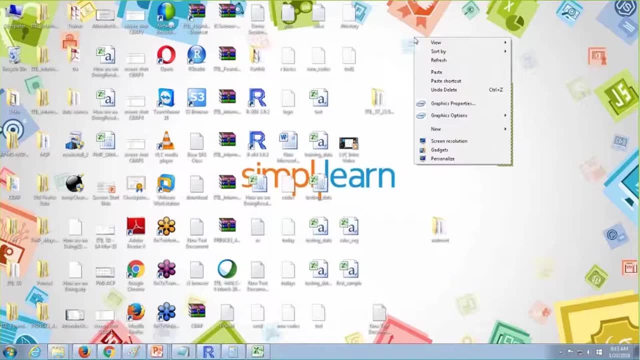 is done. ok, So this is the data set that I am going to take. I will show you how a small example in hierarchical clustering. So I will take a big data set, because for hierarchical clustering, I think these data sets are small and there is no real time data set which is available in our LMS. So what? 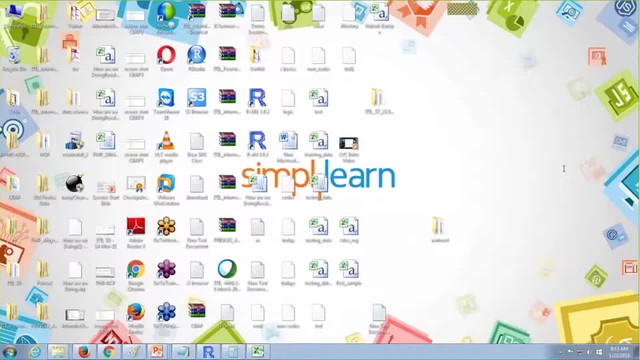 I will do is I will take some business case studies, which I have right now. I will just show you one small example in hierarchical clustering, and then on we will get into the time series part. So what is time series analysis where it is being applied? So first, 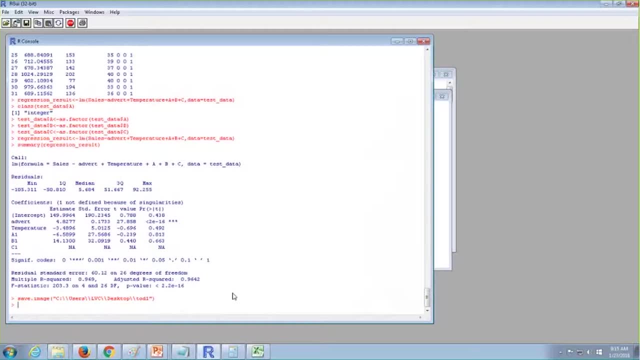 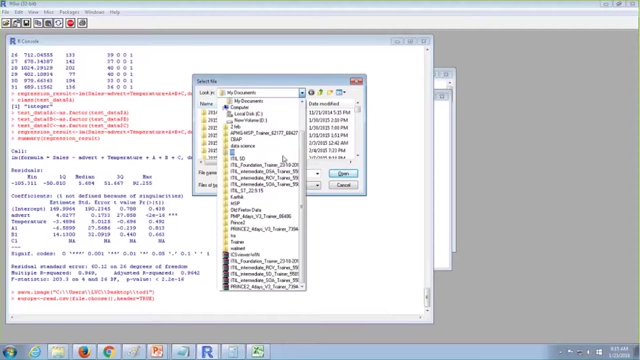 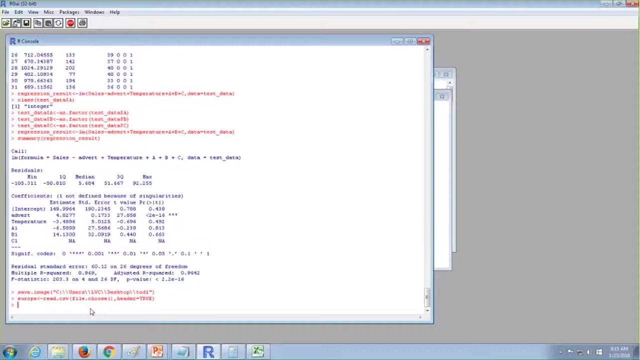 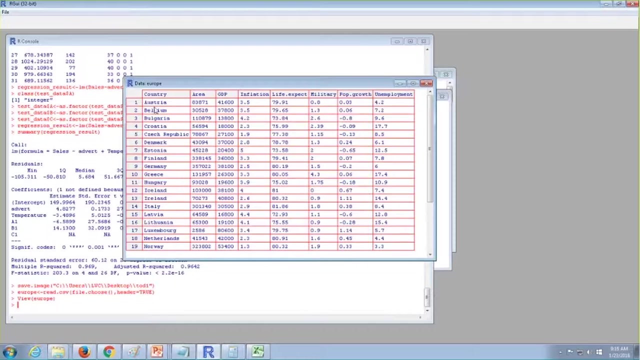 I will just take this particular data set. Ok, I will just view this particular data set. Ok, this is the data set that I have taken. Ok, Ok, Ok, Ok, Ok, Ok. So this is the data set that I have. So, probably, if you are looking at this particular 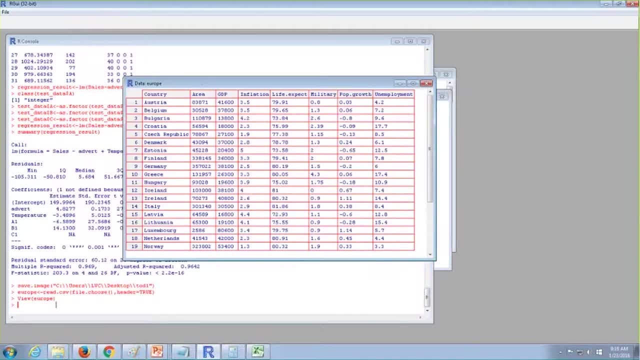 data set. I have a field called country. there are different countries and there are some of the data which is being given as area: GDP, inflation, life expectancy, military population growth and unemployment. So these are all like a quantitative variables for this particular country. So there are different countries and we will try to see how we can. 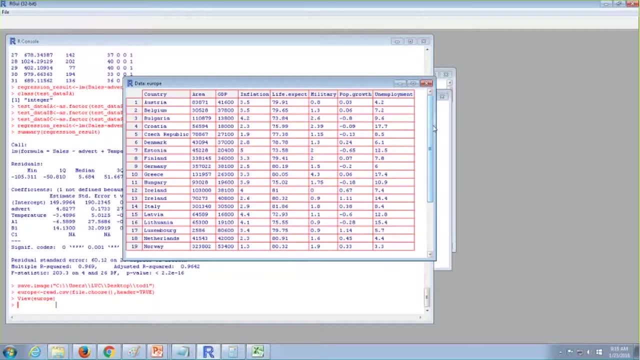 group all these countries, and what are all the countries which is having similar properties? So some of the some of the countries would have similar properties, like their area would be same and their inflation rate would be almost same. So we will try to see how this. 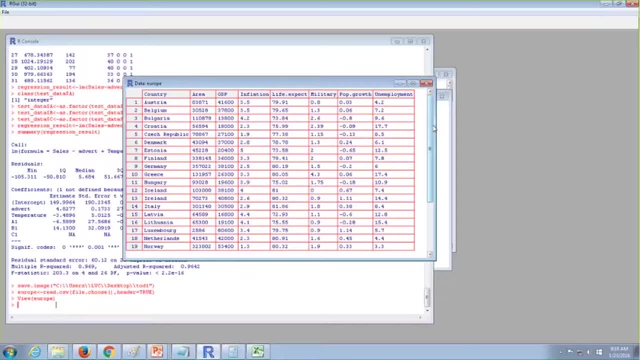 hierarchical algorithm, like hierarchical clustering algorithm, how it works in this particular data set. that is what we are going to look here. We will try to see this particular process in terms of R. So, in order to do, in order to do, k means what is the function that we 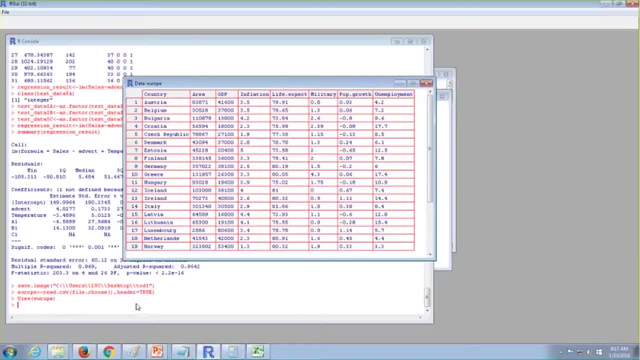 use. When we are looking at the k means example, what is the function to calculate? k means clustering. What is the function to use? k means clustering. The function is nothing but k means. So k means if you are giving a data set, then automatically k means ah clustering. 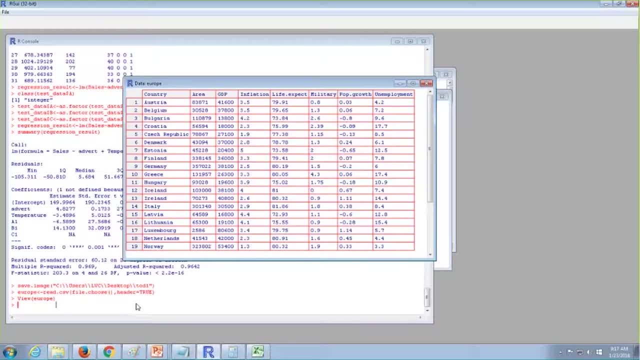 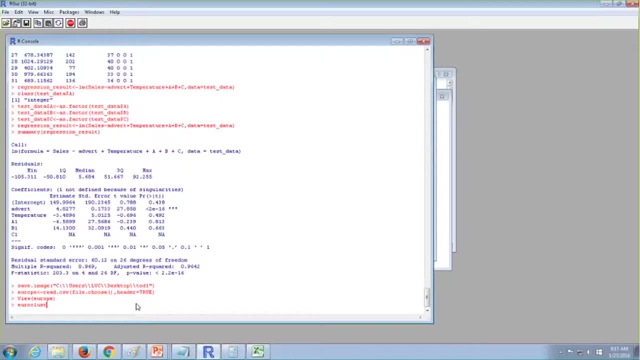 can be done In the same way. if you want to do a hierarchical clustering, the function is: I will create a variable. This is the function to calculate your hierarchical clustering and I am going to calculate based on the distance. ok, I am going to type distance. 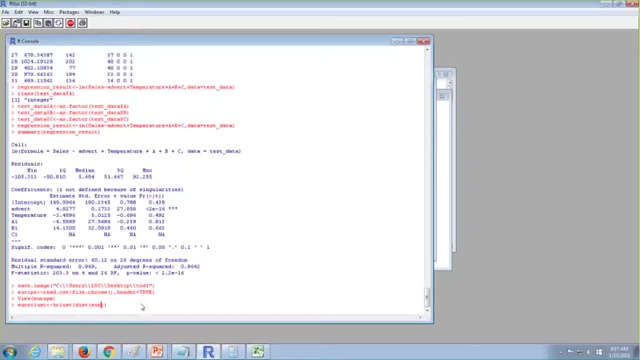 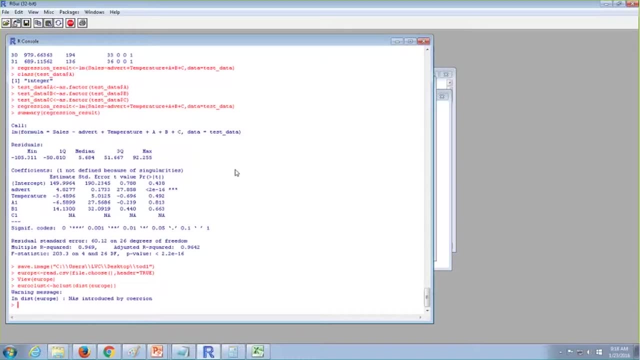 and I am going to take the data set as euro When I run this code. ah, now I would get an error. I will tell you the reason. because in my particular data set I have the first column as my categorical variable. So I have to remove this first column because the first 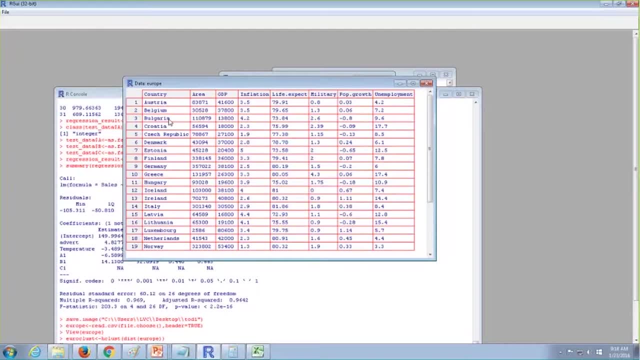 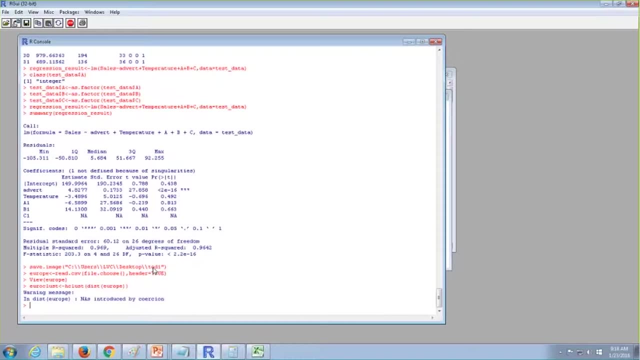 column contains all the country names. So this cannot be ah done in terms of a clustering. So what I will do is I will just remove the first column- countries. ok, then I will do the process. ok, in this Europe. I will just remove the first column. So this is the function. ok, what is the difference? 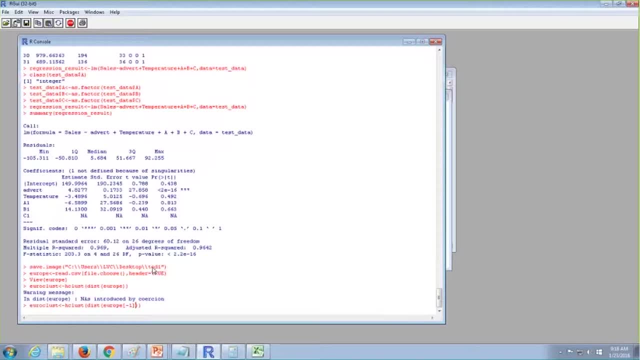 between these two types of clustering. So in terms of k means clustering, if you know the cluster size that you need to form for an example, if you know if I need to form only three clusters there, you have an option of defining your cluster numbers. that is the. 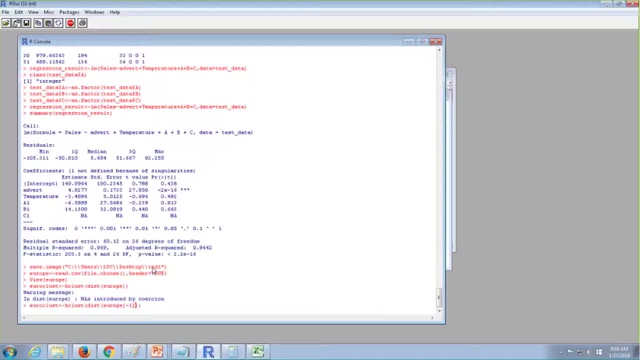 advantage of k means clustering, But when coming into hierarchy, clustering your automatically. your algorithm automatically tries to split your data points until it can get deviated. ok, So what is the maximum limit that it can divide? it can, it can do the process. So 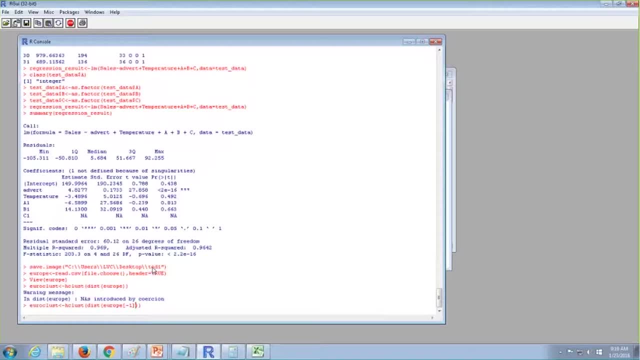 here you cannot tell that only three clusters I need to form or four clusters I need to form. that you cannot tell in hierarchy clustering. So hierarchy clustering is actually having a divisive property. So from an entire cluster it try to divide it, it will try to split based. 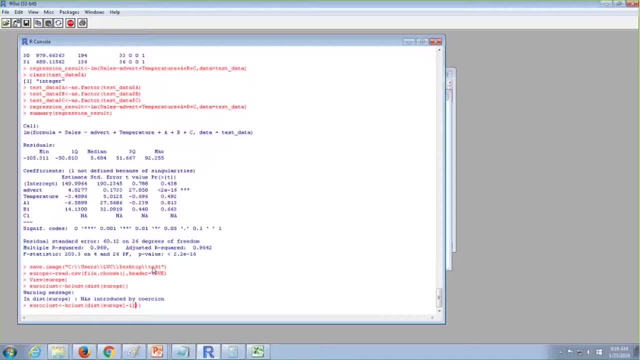 on the distance. So the distance is large. it again splits So these particular things, it it keeps on going. So at the end of the day you cannot find how many clusters that you want, but after finding a hierarchical cluster you can just see what are all the countries which. 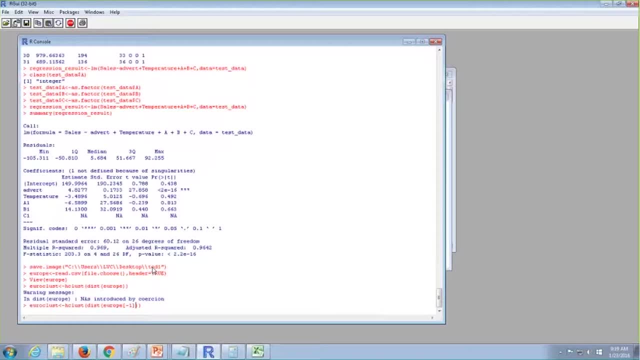 is falling in a separate group, after doing a complete hierarchy. after that you can define what are all the cluster that you are going to take. ok, ok, ah, in. in a process of clustering you can never use a categorical variable. ok, Only numerical variable. So only with numerical variable you can calculate those distances. 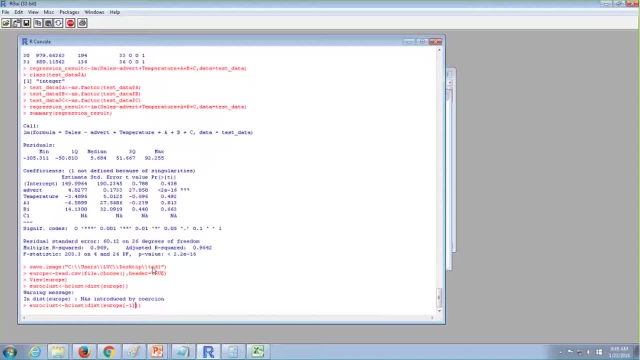 So even if we are coming ah, if you are taking a categorical way variable, and if you are ah, if you are converting as a dummy variable, that will not make any sense because even ah in in that particular case, clustering is not that effective. ok, So in those sort of situation generally people do not do a clustering, they will go for a. 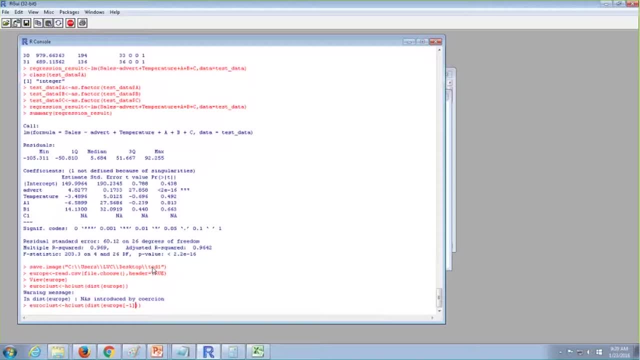 decision tree and, ah, I think decision tree is not given in our curriculum, but somehow, if I get time, I do not have time, So let us call that Again: set. so this is quicker path and smoothness: ok, So you can reach those. note temperature and then, if you move to that, 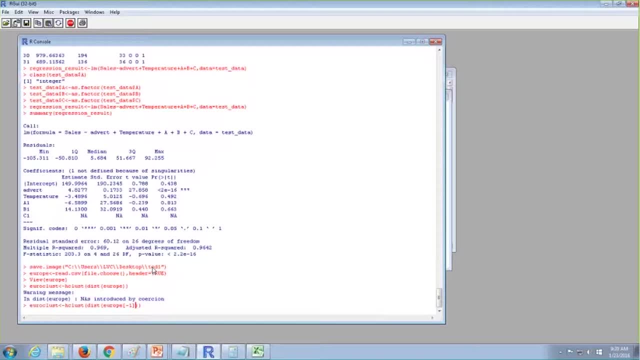 set, then the result is that you can reach to that result, Andét So I will- to get a pickle- currently those Bowseri zucchini- to that ever. allowing me toMore how, if I get time, I will also talk aboutdecision trees as well. ok, So I think, at leastif I. 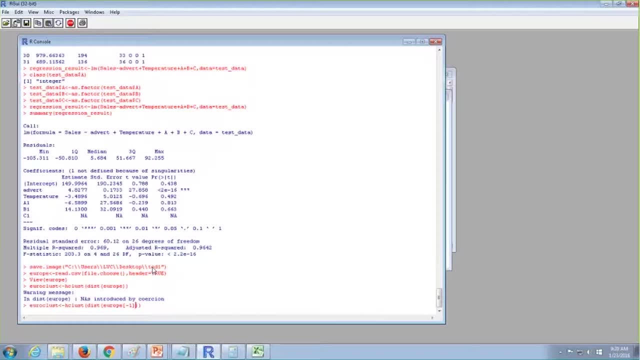 am not able to cover the entry syllabus, I will. I will at least try to give a hint about decision tree and how that particular approach is done. ok, So there in decision tree, what you will do isyou can define yourfinal dependent variable as a category and you can see what. 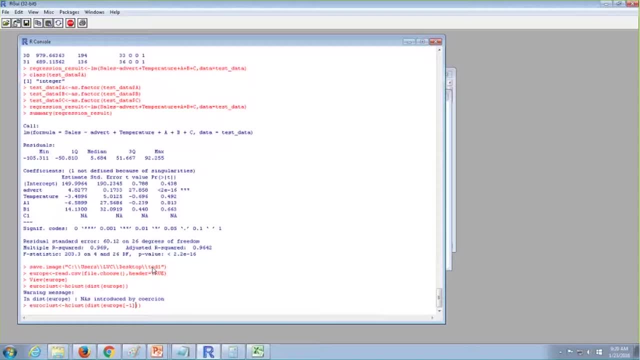 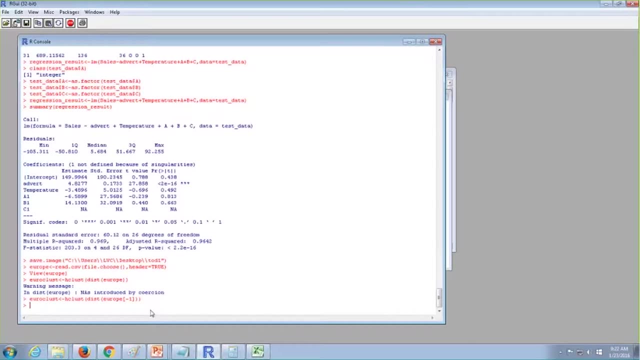 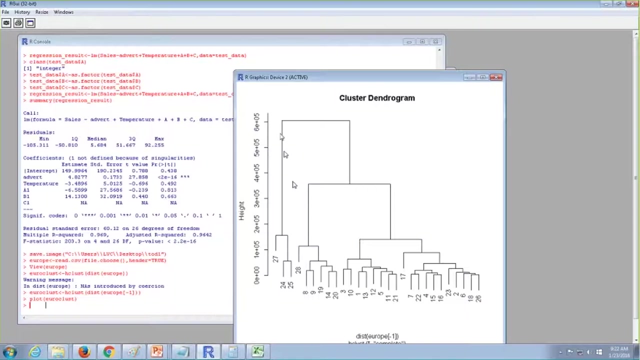 are all the parameters, which is causing to reach the entries. that is what is all about decision tree. So now, in this hierarchical clustering, I am just removing the first column. now my clustering is being done. now I will try to plot the cluster. Now, if you are looking atthe hierarchical clustering is being formed, but I think it. 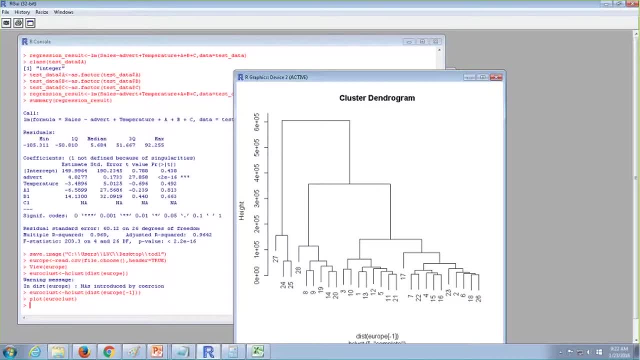 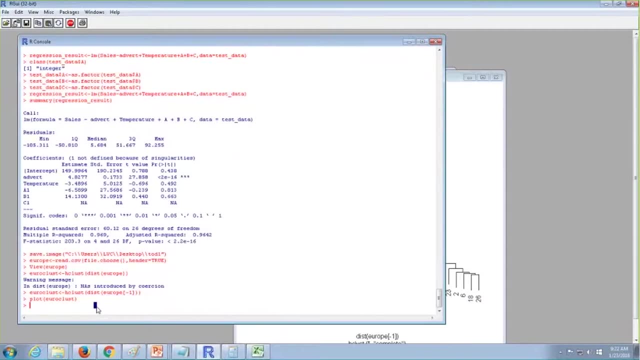 is bit difficult to understand, for what? So what I will do is, instead of these labels, I will give mycountry. So how do I do that? So how these countries are being divided, So I am just going to add a label here to: 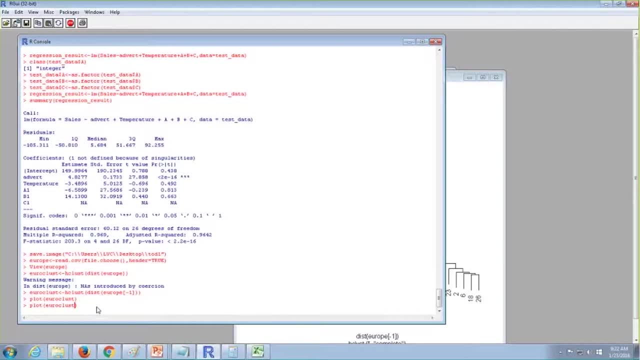 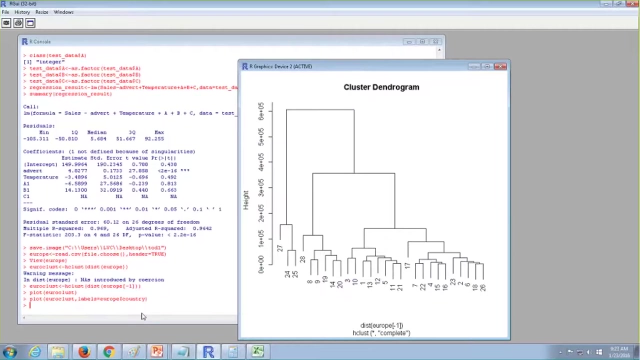 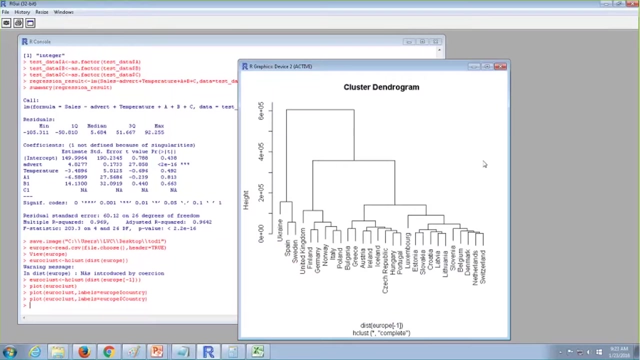 my plot. So in this plot I am going to give my labels. Now, if I include a label to my clustering that I had made, Now I can see that I have a cluster. Now I can show how these countries are being clubbed together. So if you are looking at 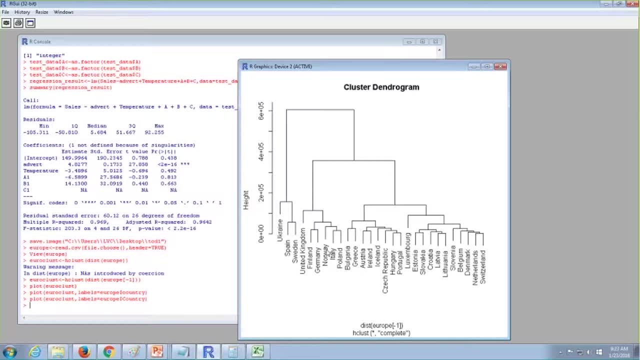 all this countries would have same properties, butin terms of k means clustering. if you know the clustering, say k is equal to 3 or something. only 3 clusters would be formed, but right now in hierarchical clustering based on the distance is. So now, if you are looking at, Spain and Sweden are having almostequal properties, and Ukraine. 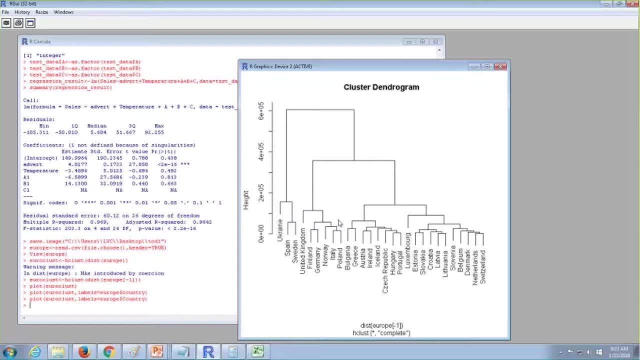 is something different and, and in this particular cluster, for an example, in the entire cluster that has been clubbed together, we had the properties. So if you look at those countries which had same properties and these are clustered in the same place, So you can see, if you are looking at, Spain and Sweden are having almost equal properties. 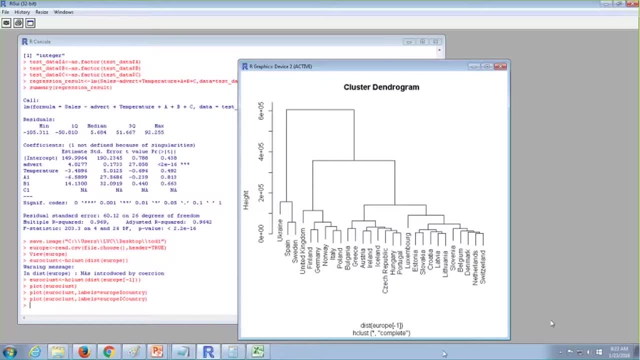 entire cluster that is being formed. if I want to form five clusters, ok, if I want to form five clusters, how that process can happen. So, after doing a entire clustering form, if you want to split this hierarchies into two or into three or into four, that process is. 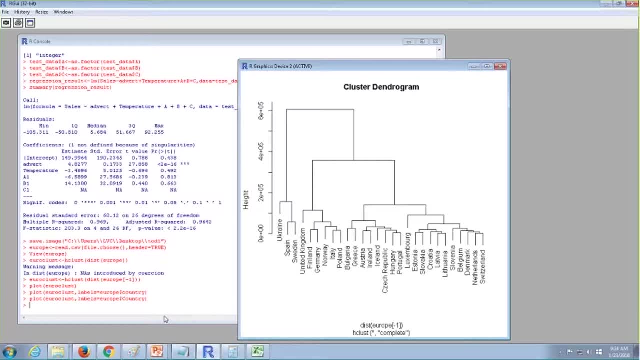 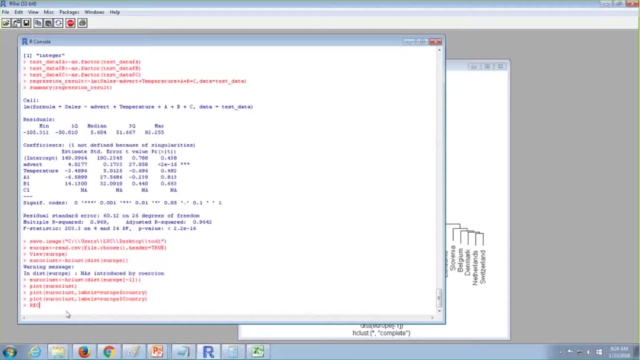 actually very, very easy to do. So I will tell you how that can be done. So there is an option called ah rectangular dot hclust. So that would give you how this clustering can be formed very easily. So, for an example, if I type rect dot- hclust, 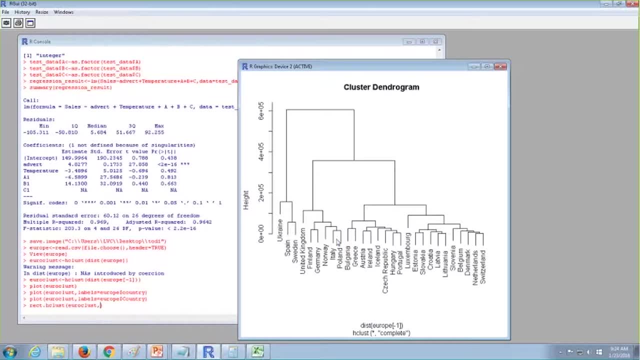 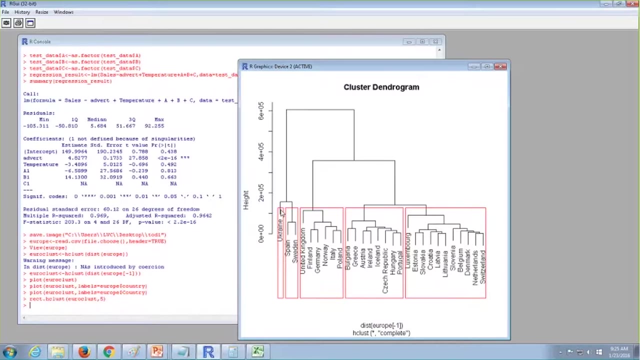 if I want to form, say if I want to form in this entire cluster which is formed, if I want to form only five clusters, I can just give here five. now, if I enter, run this code, now I can see how this five clusters are formed. So Ukraine is something which is different, which is having the ah extreme. 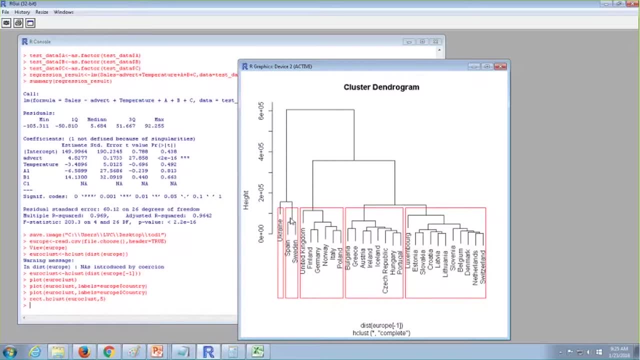 distance. So these points are having closer distance when comparing to these clusters. So this is how the clusters can be divided. now we can tell if I need to form five clusters. ok, ah, Bulgaria, Greece, Austria, Ireland, and everything is falling in a particular clusters. 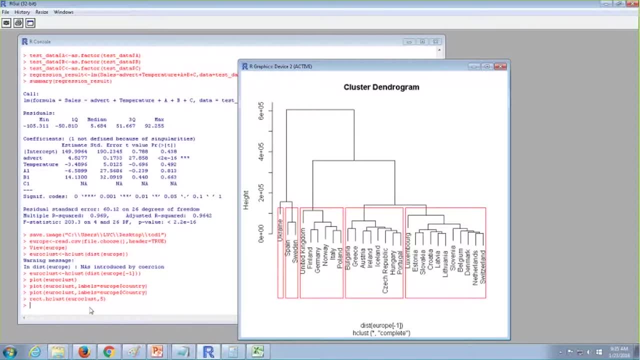 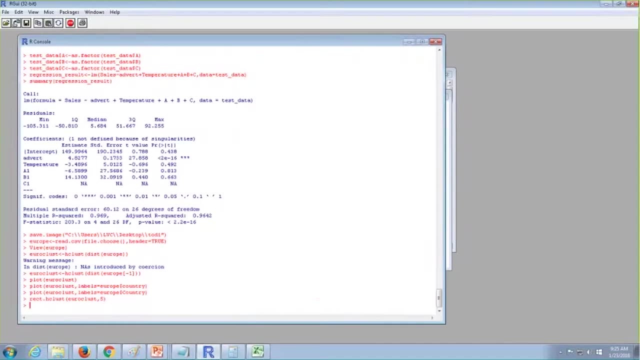 So you can just go ahead with this particular process, ok. and if you want to change the cluster numbers, like say now after forming the entire cluster, if I want to form only four clusters, that is also easy. So first I will again I will run the script. ok, now if I want to. 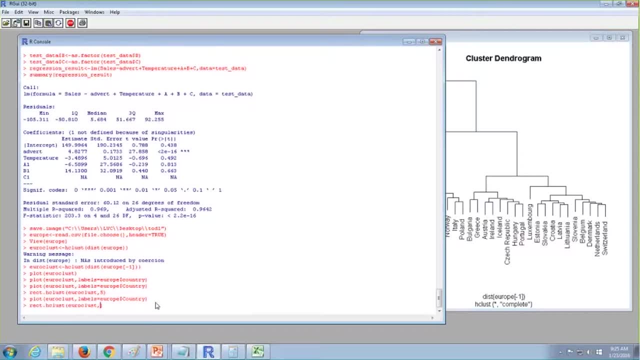 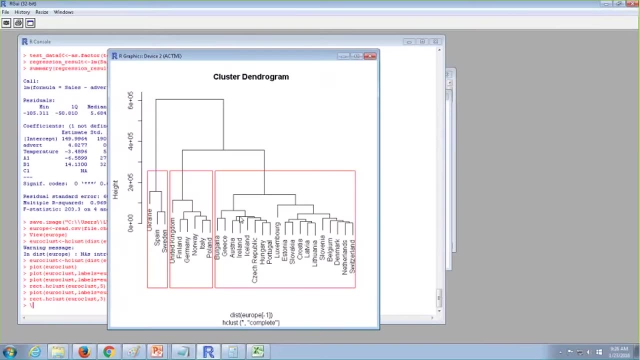 form. last time I have formed five clusters. if I want to form only, ah, three clusters, ok, now I can see, based on this distance, now I can see. ok, these are all the clusters which is having closer properties And this is binded together and formed as a particular cluster. and this is the second. 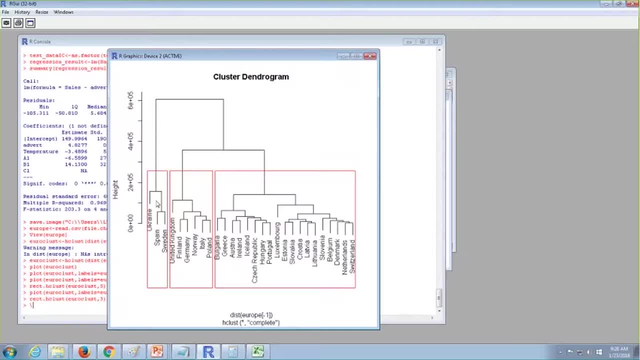 and this is the third. this is this is how we are hierarchical clustering work. So hierarchical clustering would divide into all the possible divisive. So till the point it reaches one, it tries to do it, it tries to divide. So this is also called as divisive algorithm. 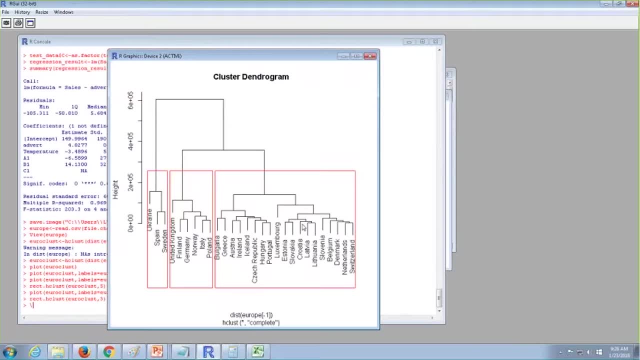 So, based on the distance, again it splits. So if the distance are close together, first there would be in big cluster. ah, based on the distance it split into two cluster and this two again it will have a branch. So this keeps on going until every, every particular country will have a single node. 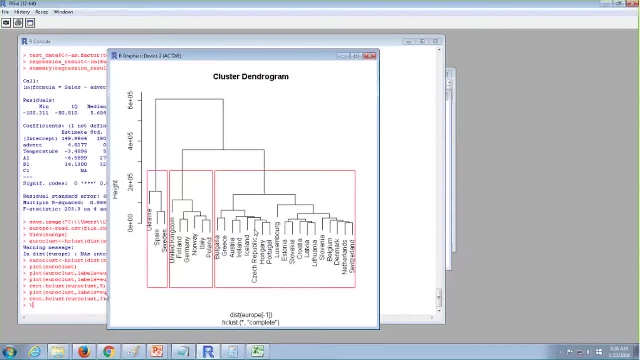 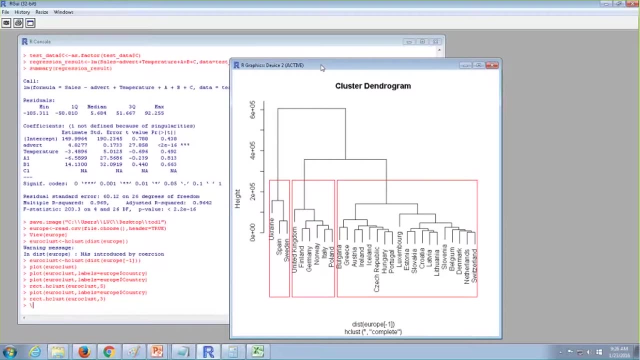 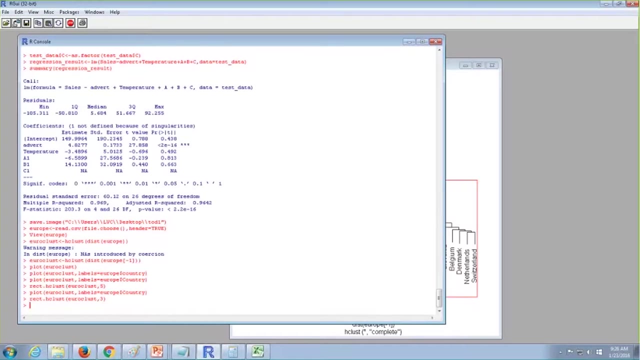 until the leaf node becomes one, this process happens and after that you can form a cluster: ok, based on the distances. ok, clear, clear, everyone. and if you, if you want to know how this particular clustering validation is done, I think, ah, for that particular, I will take a, I will take. 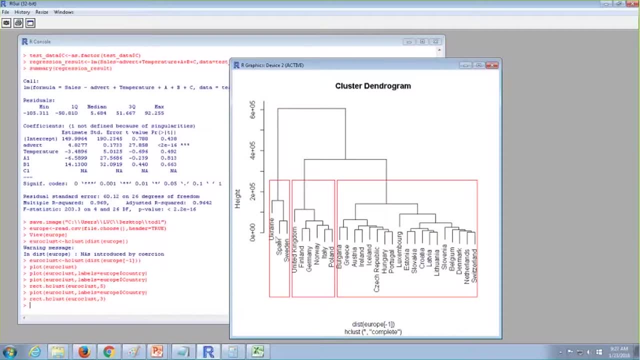 some other example in terms of a business case, because here, ah, latitude, longitude and GDP, ah, this numeric thing will not give you a good business insight. But when coming into a business insight, what I will do is I will show you some of the data set. ah, I will take hundred stores which has different properties. say, one store would have 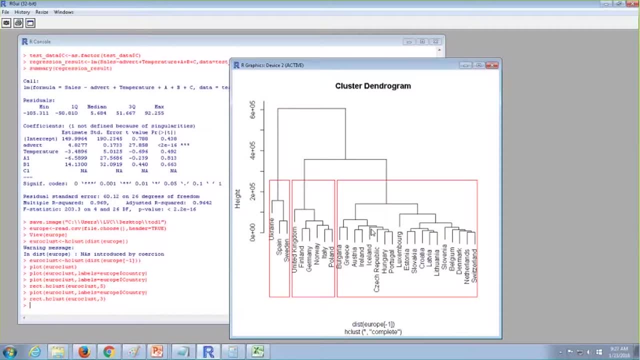 higher sales, and product mix is something different, and price incidity. So I will create a table in such a way that it has different properties. So, based on that particular data set, we will see how the validation happens. So, for an example, if I am going to include 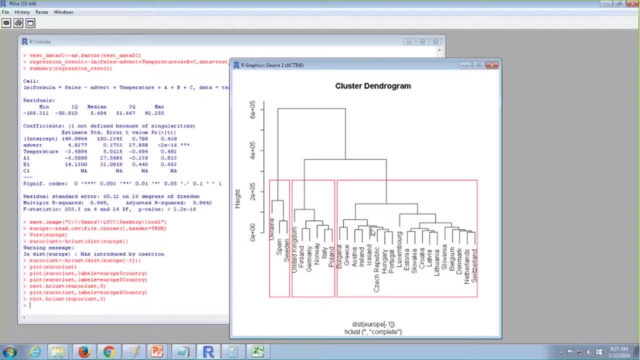 a new member into the cluster. to which, ah, to which cluster does this particular member belong? ok, So those sort of situations, I think, ah, tomorrow I will show you an example how those process would happen. ok, The last two hours, ah, when I take a real time example, I can tell you how this particular cluster is validated. ok, 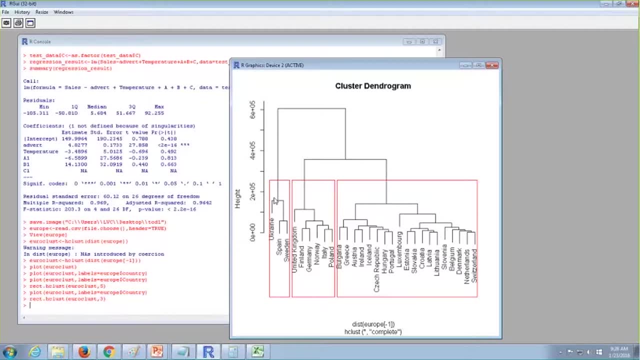 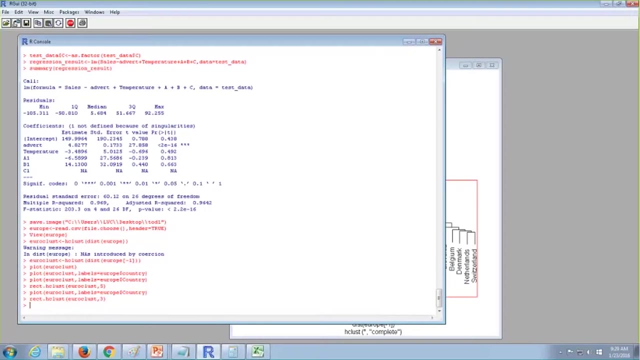 ok. So they ask me a question: what is the difference between K means and hierarchy clustering? ok, So when I do a process of k means clustering, So I think I will do the same here in k means- I will show you for an example I will take this data set: what is the function of k means. 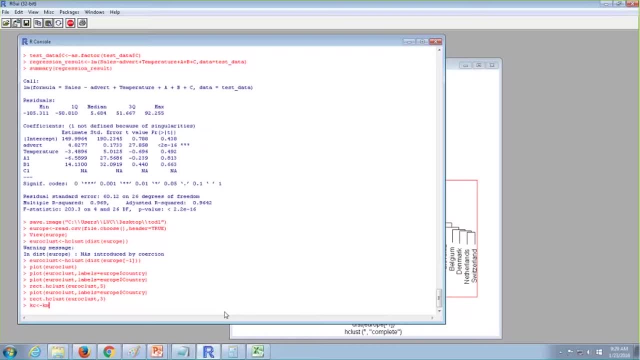 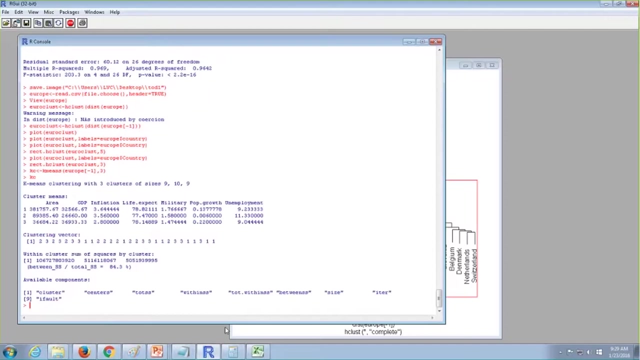 So k means is nothing, but this is a function. instead of h plus, you need to do k means, and I will take this same example, and what I am going to do is I am going to form three clusters here. ok, Now, if I see how different countries are splitted into three clusters, this is the 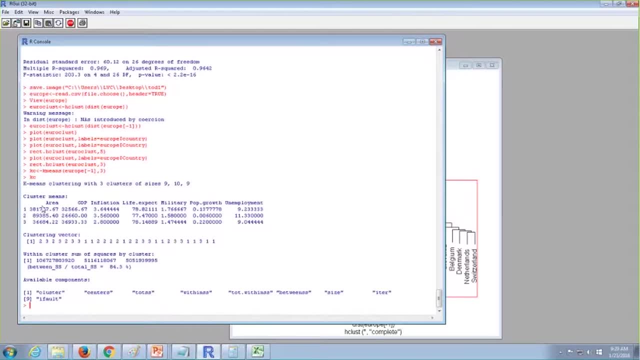 way it is splitted. and these are all the cluster mean. So for the first cluster, now you can tell that, ok, My first cluster would have a average area of 381757 and GDP of 32566. ok, and inflation on, and all these parameters are being given. So based on this, the clusters are formed. 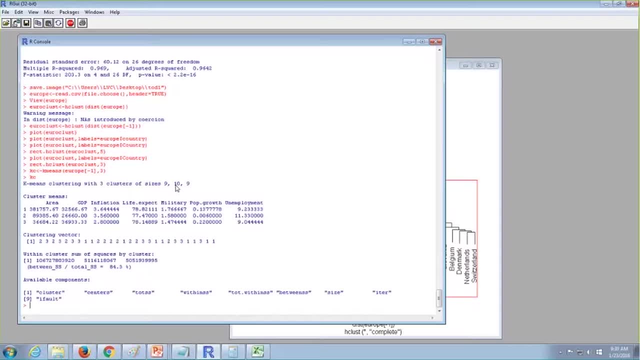 right now my cluster size, if you are looking at my total count is 28. there are 28 countries. these 28 countries I have splitted into three different cluster. Now I can see this is the purpose of k means. So whatever cluster size that if I that I define, I can form that. 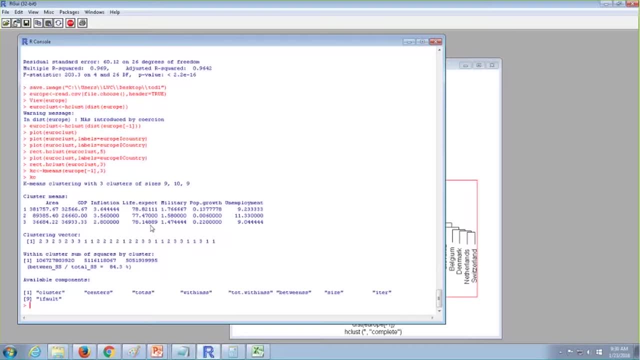 number of clusters. So if you are very sure that, ok, your end result should contain only 4 cluster or 5 cluster, then you can go ahead with k means clustering, but you are not very sure that how many clusters to be formed. For an example, when you do a k means clustering, just assume that the two 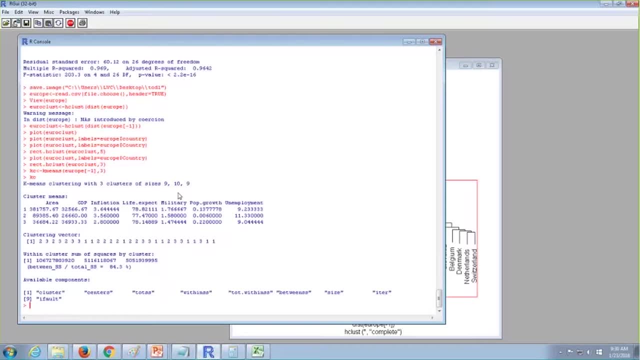 clusters. right now it is very small, but assume that in a, in case of a large number of data, you form a. k means clustering with cluster size of 3.. In one cluster you found 100 variables. in second cluster you found 100 variables. in third cluster you found 100 variables. 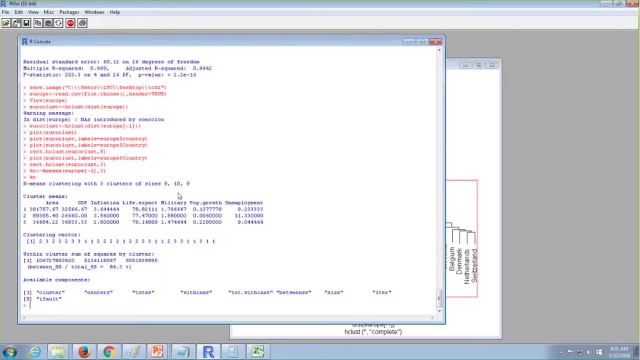 in fourth cluster you found 100 variables. in fifth cluster you found 100 variables. in the second cluster you found 100 variables, and in the third cluster you found 900 variables. ok, So totally, I have thousand as my data point. So one cluster had hundred, the second 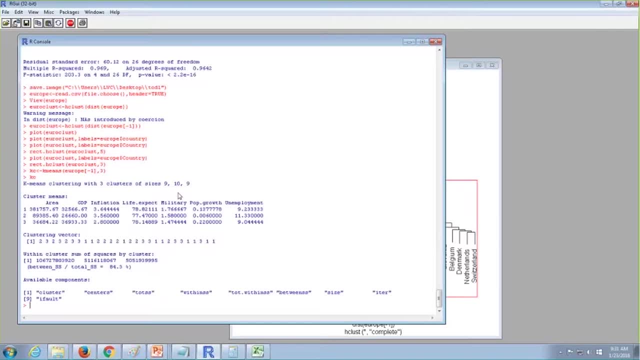 cluster had 100. third cluster had 900. ok, this three ah, but with the three clusters I cannot have any clear business decisions right? For an example, in my third cluster there are almost 900 stores. So I do not know how my 900 store is going to behave in my third cluster. So 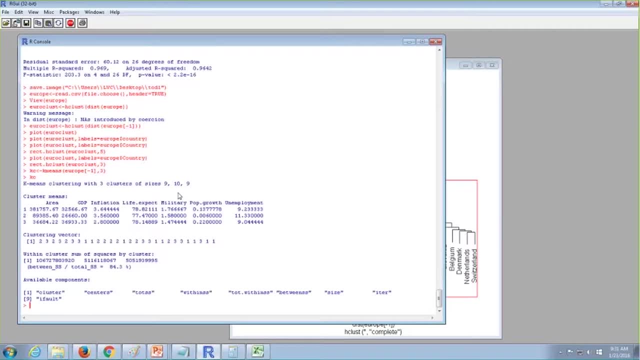 So again, what I have to do is again the third, ah, third cluster. again I have to do a k means or I have to do a hierarchical to split that in a further way, right, But when I do a hierarchical clustering directly, I can see how these branches are formed and how, how the distance are being. 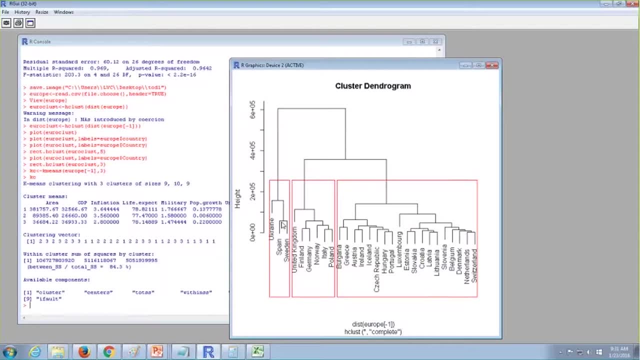 ah, equidistant, So how it is being easily divided. that is the whole purpose of k means and hierarchical. So k means you can define your cluster number. So if you want only three, you can just define three, but you cannot have any equal distributions there. ok, So 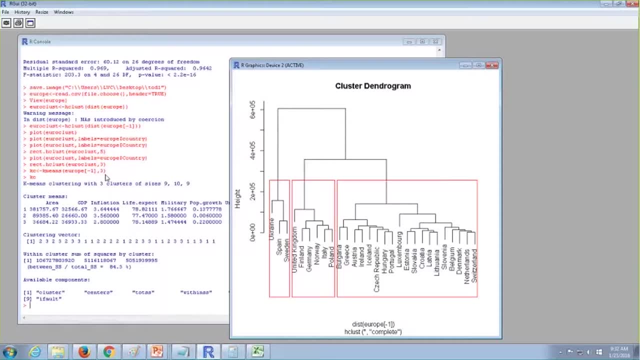 if you know very sure that this is the clustered size that I am going to make, then you can define. k means clustering, And if you are not very sure about the cluster size that you are going to form, then you can go ahead with hierarchical clustering. ok, clear, ok, ah. 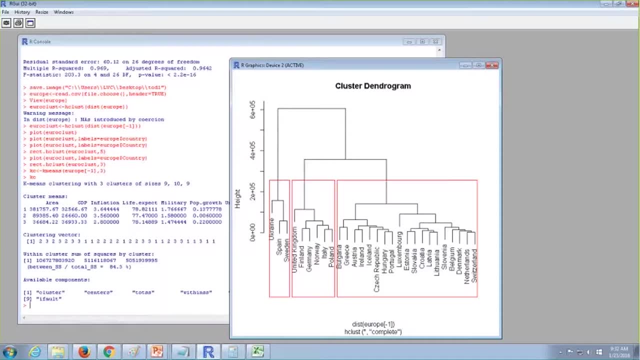 why I had given e row minus 1.. So my first column is actually country. So if I display e row minus 1. So if I display e row minus 1. So if I display e row minus 1. So if I 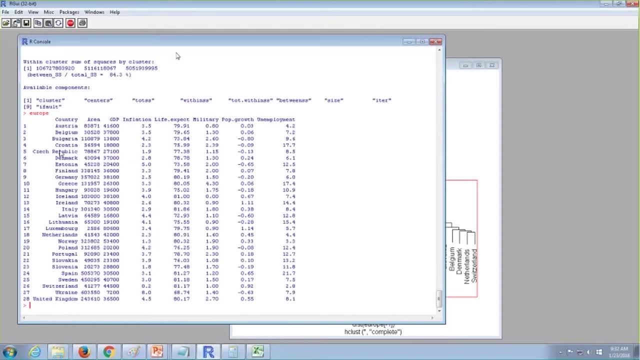 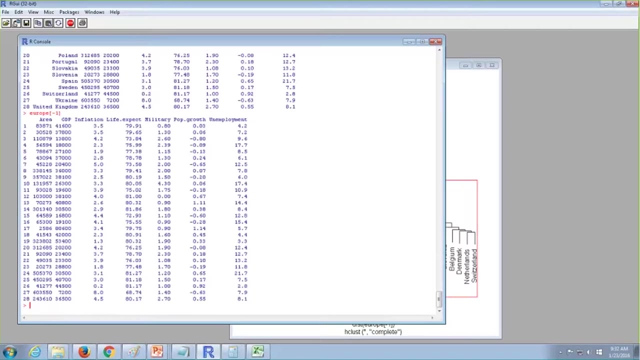 display e row. I can see country as my category, So the first column is country. that is why I had removed my first column. So the ah, the option to remove first column is e row. if I remove minus 1, I can see my first column, which is country, is being removed. ok, that. 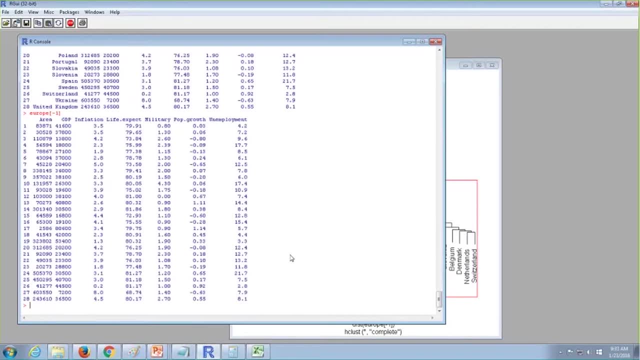 is why I did this particular process. ok, ah, In this case, do we have to look at if the data is normally distributed or not? ah, It is not necessary because, ah, it is not necessary because, ah, even if you have an out layer, for an example, can you just tell me, ah, in. 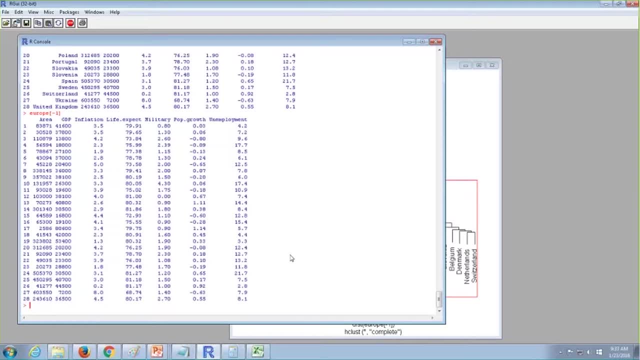 what sort of situations you can do a clustering. So I simply I did a cluster. So what are all the advantages of doing a cluster? ok, We need to know how elements in data set behaves- yeah, that is one thing- and how your data sets are associated. So what are all the properties? 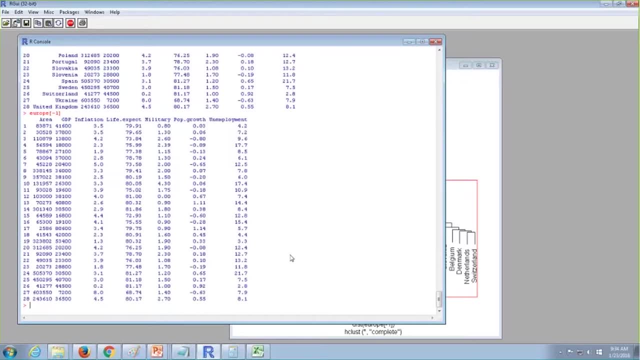 which is binding all those data points together. that is one thing And the other thing is, for an example: ah, even I can think this cluster could be a cluster, So I can just look at. could tell me what is an outlier right? for an example, if I have some outliers in my dataset? 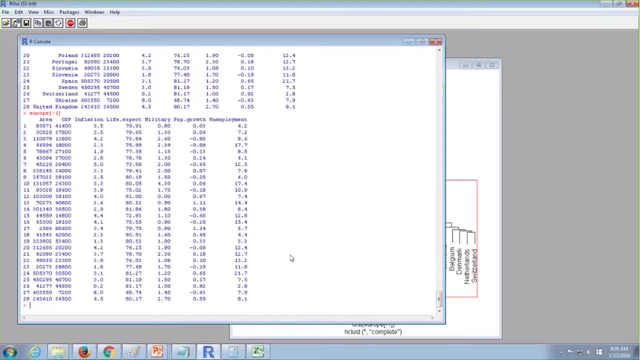 even this clustering technique can tell me what are all the outliers and what are all the stores which is behaving in an odd way, or what are all the parameters which is behaving in an extreme level. even that I can do here right, because clustering is nothing, but if 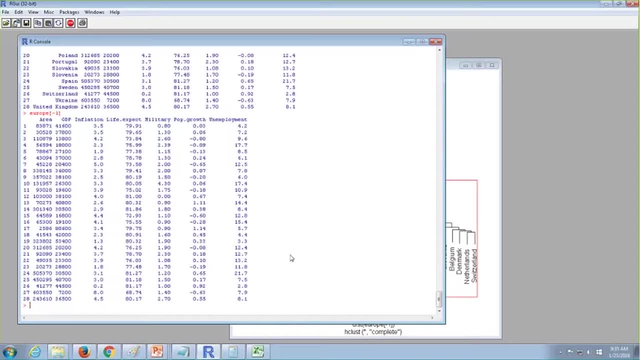 your distance is more, again it will fall a separate cluster. so based on this I can also find what are all my outliers right easily. I can also do a outlier process using clustering. so if I want to see, okay, if I have everyday sales, or I think that, okay, I have thousand. 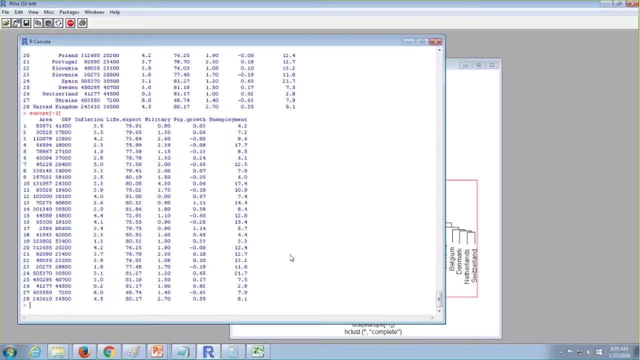 stores. in thousand stores, one or two stores would have extreme sales. so according to us, that cannot be an outlier, but that is actually an extreme action which is happening. so in order to do or in order to predict that sort of unexpected behaviors, even you can use this. 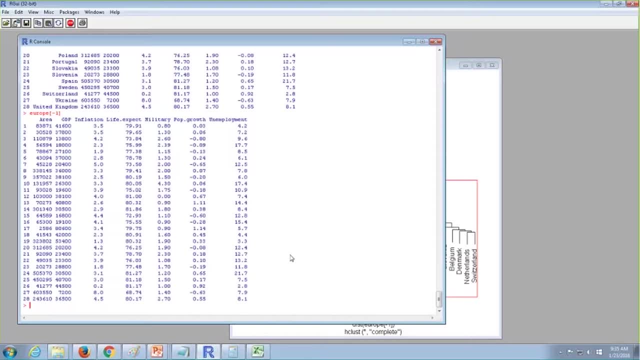 clustering to find that, because everything is all about distance right. so clustering is nothing but a simple logic where you are calculating the distance right and you are calculating the distance between two points. if it is having, if it has minimum distance, then they are binded together and they are formed in a single cluster. if the distance 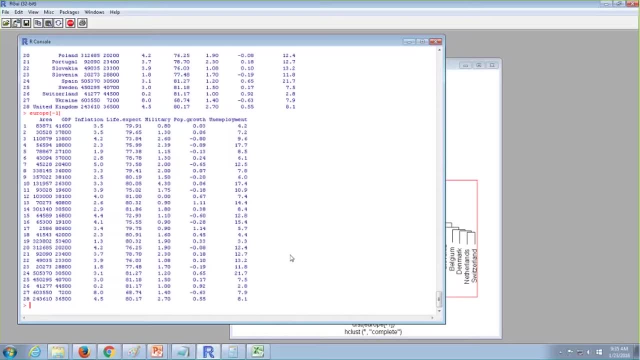 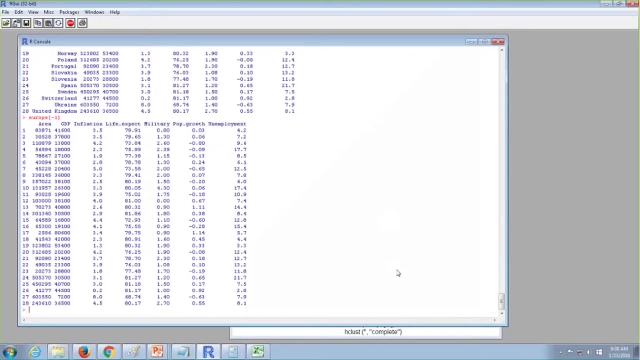 is more they can fall in different clusters. okay, that is the whole point of clustering. so cluster validation and all these things, I think with this small dataset we cannot work on this validation part. what is the practical use? okay, practical use in the sense generally why we do clustering is in some of the cases, generally client would have a doubt. okay, I. 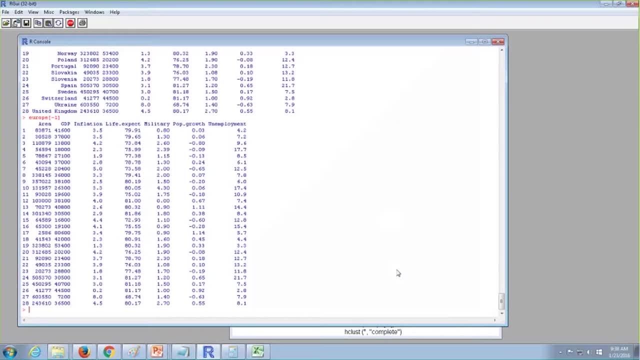 am going. I am going to take certain decision. so, for an example, if I am going to take a promotional decision, okay, I am going to implement some promotion. what are all the stores should I do a promotion and in what are all the stores should I not do a promotion? if I do a promotion, what is? 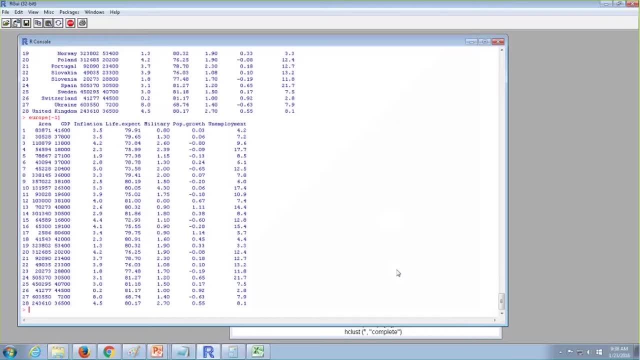 the promotion level that I can do. for an example, if you consider Bangalore, like there are some places where people are not that effective towards price, even if you are making a promotion there, it will actually like a normal sales would happen, because people would not very okay. so those people are like high standard people, so what they'll do is, even if it is, 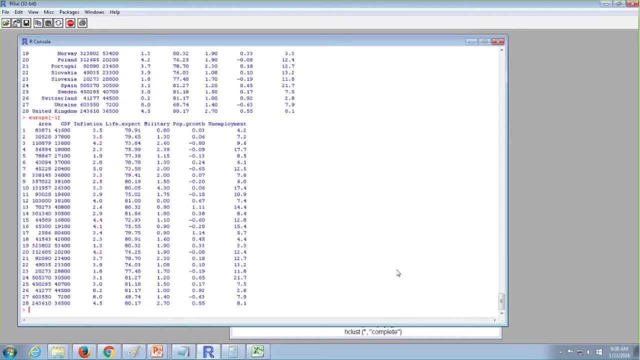 promotional day or non-promotional day for them, actually, that is something normal. so whenever a company is going to take a promotional decision, right, they would always think: where should I implement this particular idea? for an example, if I, if I am going to give a 30%? 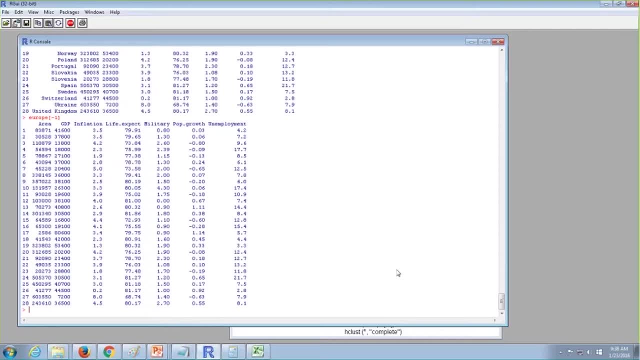 off on a particular product? should I give 30% off on a particular product for every store that I have or for a particular store that I have? so they should take all this decision. so all this decision We could Suggest them based on this clustering behavior, so some of the cluster, if you're looking at. 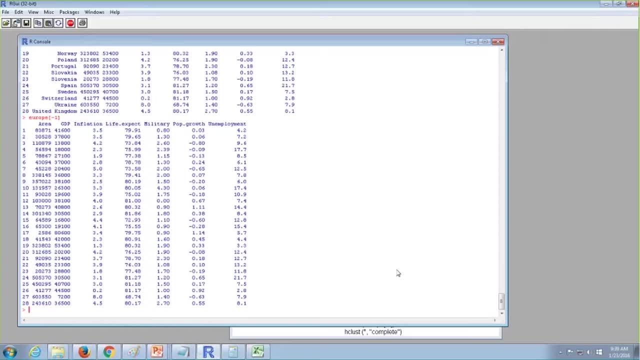 you can just see the product is going down. the reason can be because of high price. so in those sort of clusters alone you can form, you can take some of your decisions in changing your business in a better way. okay, or as a or as another example, if you want to launch. 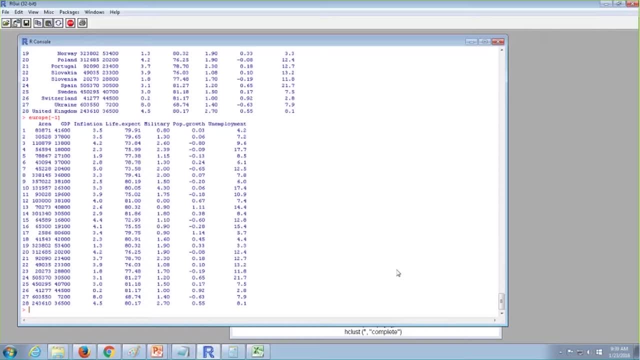 a new product. so in order to launch a new product, I need to know what are all the stores that is performing well, Which could Readily accept an innovation product or which can readily accept a new product. so those sort of stores I need to pick up right. so those things you can do with terms of a clustering. 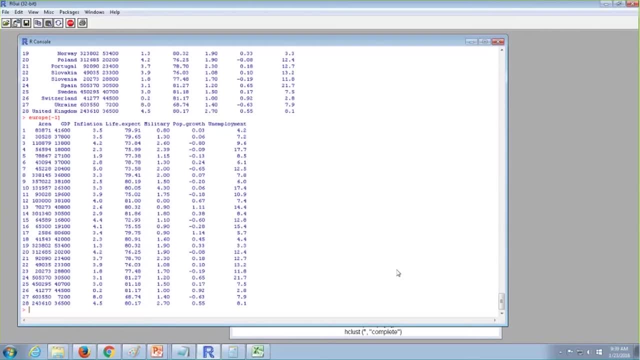 and some people also will try to see how the in terms of store segmentation generally, people would look clustering in terms of a store segmentation or a product segmentation and even for a outlier detection also, sometimes people would use clustering. so these are all the practical examples. Generally, 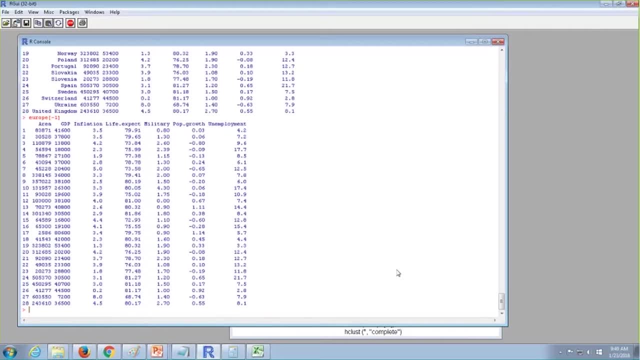 Generally, people would do all this process. okay, and I think you asked a question: what? what are all the other clustering algorithms available and which one is the best? for example, there any algorithm which would be effective? okay, so generally, if you're looking at clustering algorithm, there are different clustering algorithms like k-means, k-means and hierarchical are the. 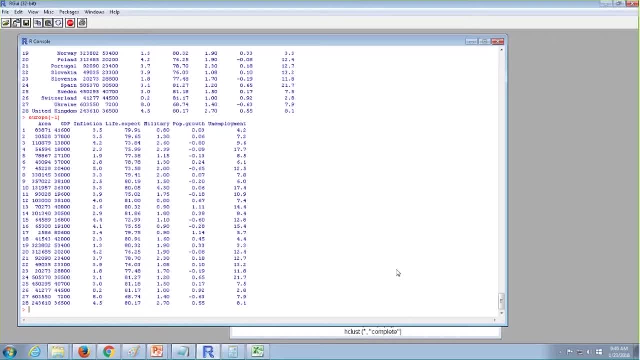 most popular clustering algorithm, that which is followed from the traditional day till this point, Generally So k-means clustering and hierarchical clustering and apart from that, like something like db scan is there and these are all the most probably. generally, people would go with only these. 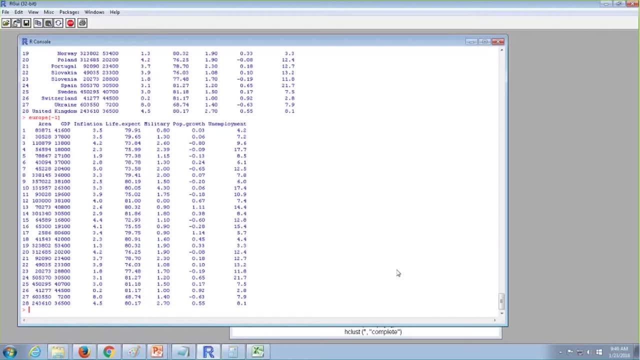 three algorithms. so apart from that, the way the distance are calculated can be different. so the only matrix that they would do is they will try to optimize their distance level. so first they will try to club all the shorter distance, or they can club the equidistance. 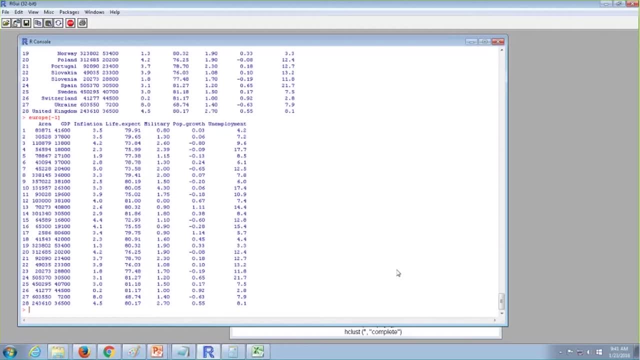 part. only the distance matrix that they choose would be different. okay, but the clustering algorithm- even If you look at some of the clustering algorithm, only the distance matrix that they are calculating would be different. so initially they will try to form a big cluster. from then they will. 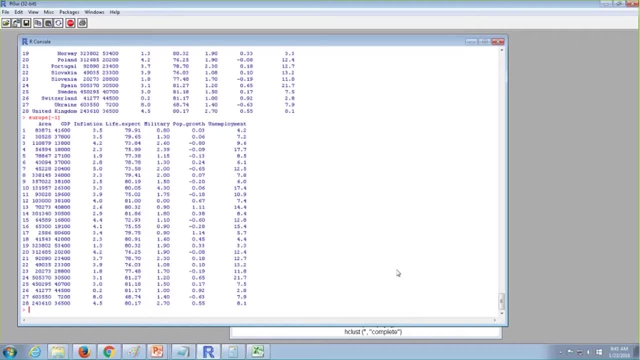 start to divide or some people. what they will do is they will start from a small cluster. they will try to club it. so in an either way it can be divisive or an agglomerative. so that is the two point that they will do. only the distance matrix calculations would differ. 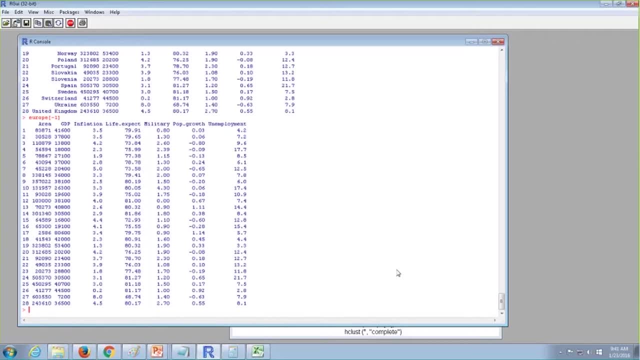 so some people, what they will do is they will try to calculate the error terms from one point to the other point If the error term is less Okay. So again, that is a matrix to calculate the distance. right, if the error is large, then the distance is large. so some people would use error or some people would find the distance. 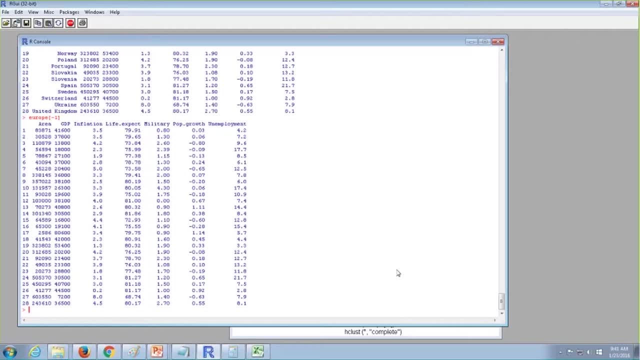 so only the distance matrix would be differing in all the algorithms. okay, and it depends. so when you are doing a k-means, and hierarchical, because that depends on the business situations, because if you have a fixed number of cluster to be formed, say, then in that case definitely. 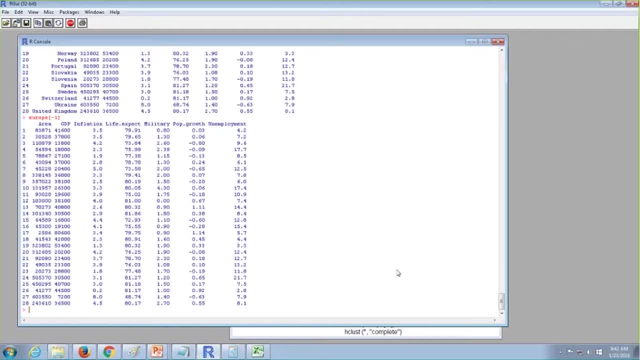 k-means would work better. So this is also like you cannot decide with clustering. so clustering is actually an iterative process. we can which you cannot fix. I can do, for an example, to fix a cluster. size itself is actually an iterative process, for an example. sometimes you would fix. okay, I want to form. 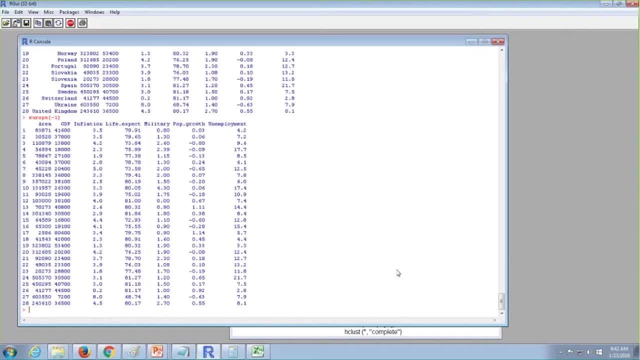 10 cluster. but after forming 10 cluster, if you are not able to find any insight again, what you will do? you will try to increase your cluster size. so that depends on the business case. so definitely, generally people, if you are asking me a question, what is the order? 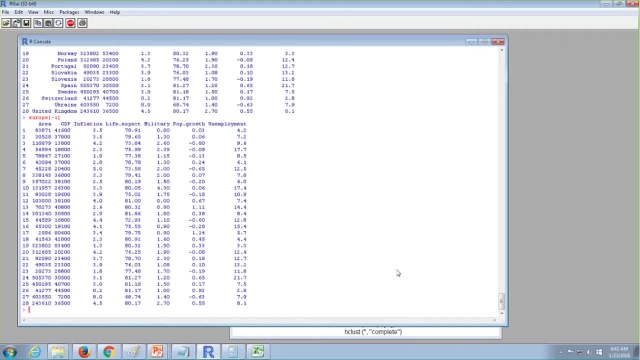 of the cluster size. what is the optimal cluster size? no one can give you an optimal cluster size according to formula. people would tell: okay, root of n plus 1 by 2, but actually in a real time way that will not work out. so in order to form your optimal cluster size, 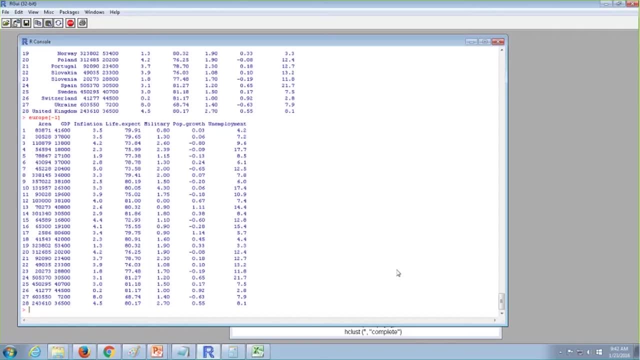 you have to under grow many iterations so generally people cannot tell that this is the cluster size that I want. you got my point right because if I fix that, my cluster size should be 5.. And after making a cluster, if I am not able to find a cluster size, then what I am going? 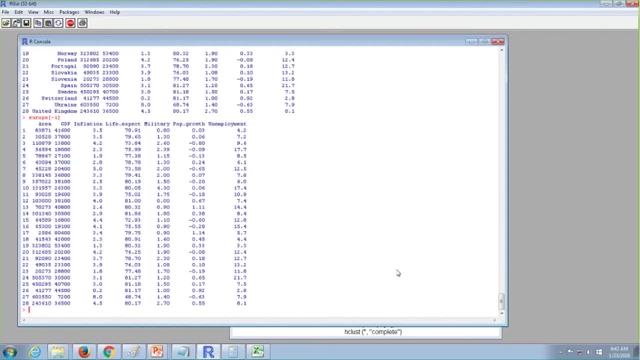 to do is: I am not going to be able to find a cluster size and I am not going to be able to find a cluster size. If I am not able to find any insight, then what I will do again: I have to change the iteration, so I have to change the cluster size. so this cluster size is something you 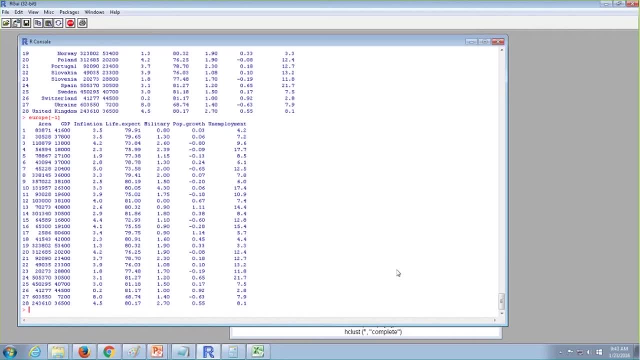 would be doing until you get a business insight. so, until you are not able to find an insight, this keeps on iterating. okay, this is, clustering is all about understanding your business right, because to understand your business you have to fix how many clusters that that you need to form. so, for an example, as I told you, I form 3 clusters where in one cluster I have 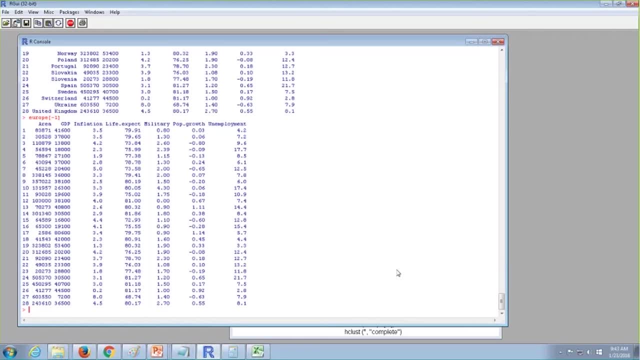 100 store, second cluster. I have 100 store third cluster. I have 900 stores. okay, in that 900 I cannot get any business insight. so what I can do is I can take only the third cluster again. I again I can try to split it to get better insight. this is how generally clustering: would go ahead.